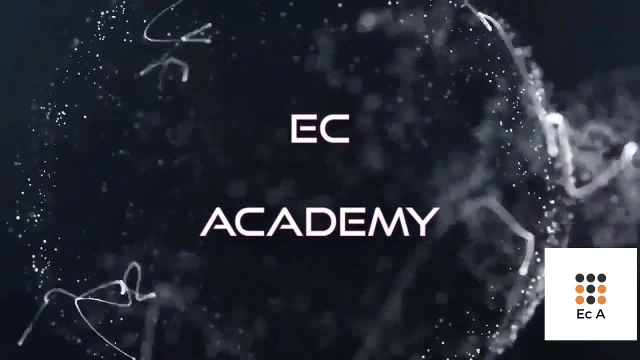 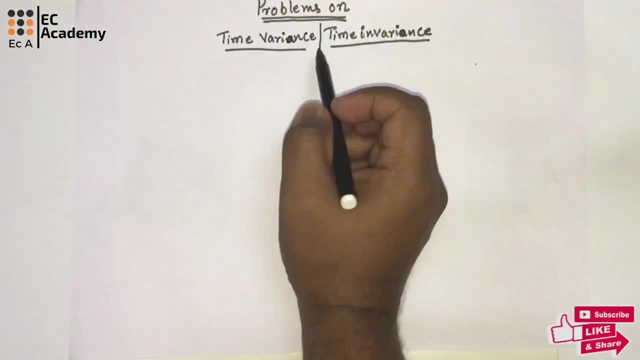 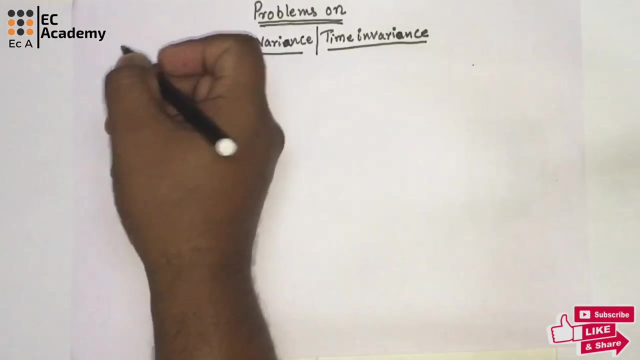 Hello friends, welcome to EC Academy. In this lecture let us understand the problems on time variance or time invariance system. A system is said to be time invariant if the time shift at the input causes the corresponding time shift at the output, which means y of t minus t naught. 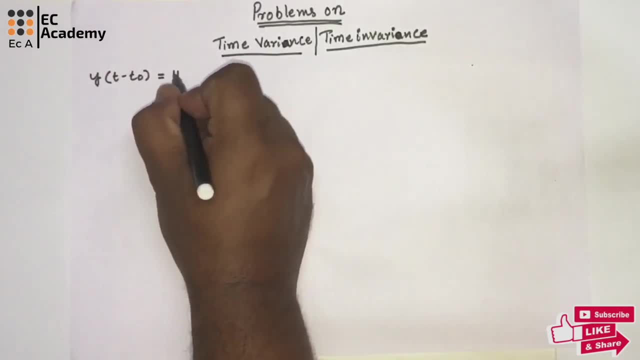 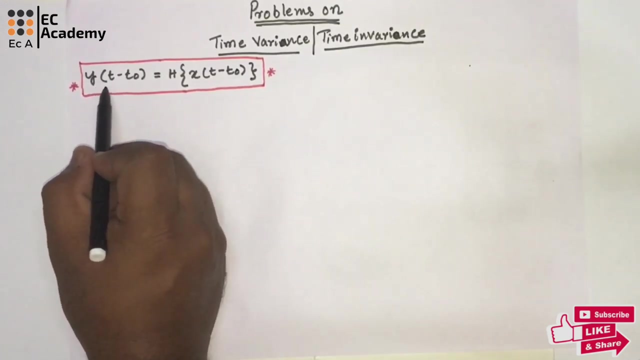 is equal to system response to the input of x, of t minus t naught. So you can see if there is a time shift at the input that should be reflected at the output as well. You can see there is a time shift at the output as well. Such type of systems are known as time invariant. 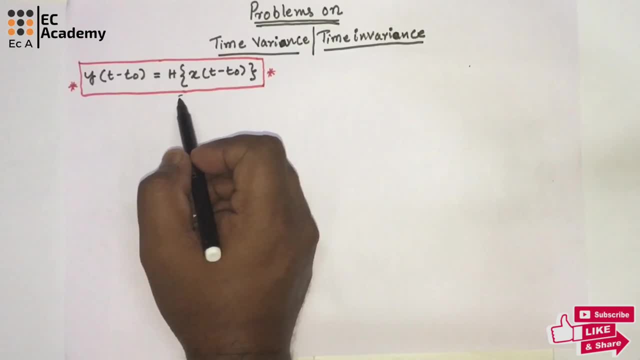 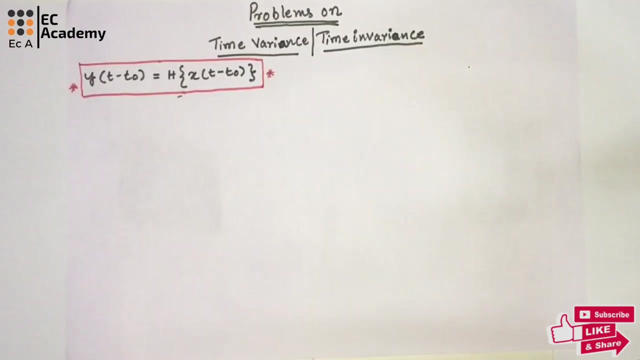 system. So if it does not satisfy this condition, then the system is time variant system. So here h is the response of the system. So the system is responding to the time shift at the input and that should be reflected at the output. So now let us solve few problem to understand the time. 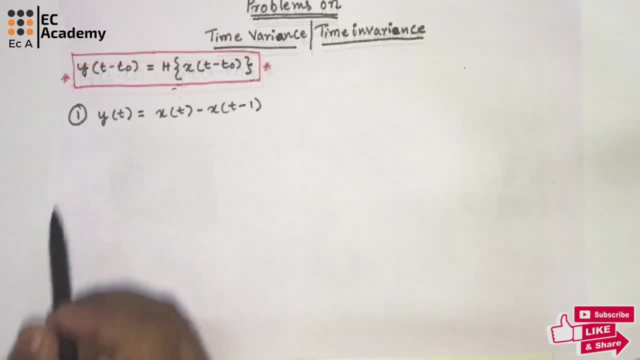 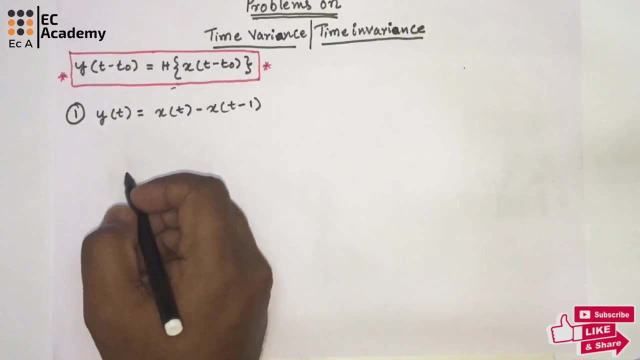 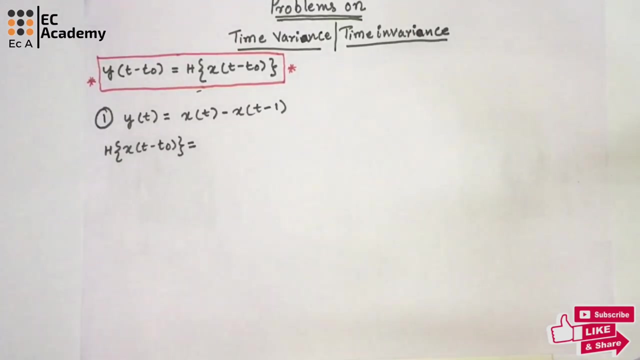 invariance and time variant system. Now let us consider the first problem, where y of t is equal to x of t minus x of t minus 1.. Now let us find the time shift at the input. So here, always remember, in the first side, we need to perform the time shift operation for t, So we can write this as x of t. 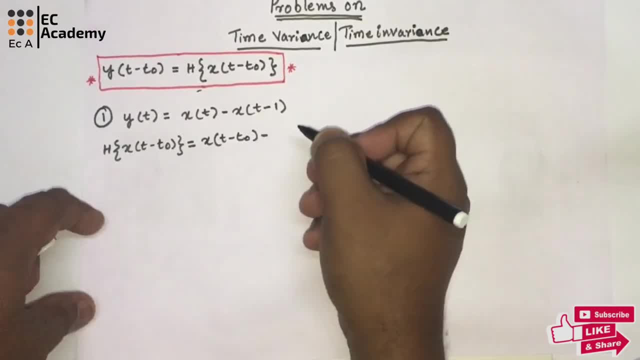 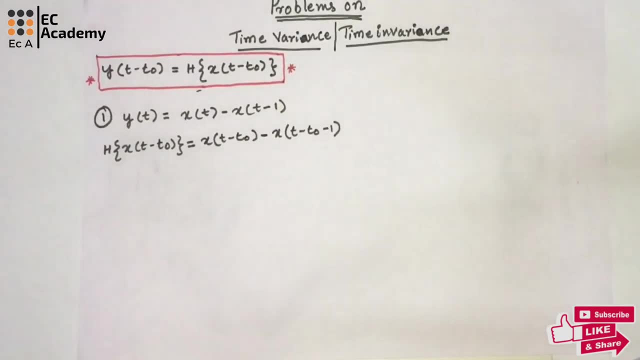 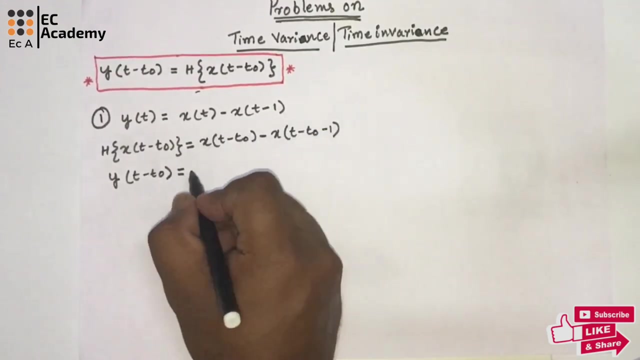 minus t naught minus x of t minus t naught minus 1.. So we are performing time shift operation at the input. If we take output y of t, so we can find y of t minus t naught. So here, always remember, we need to replace t by t minus t0.. So let us take the equation. 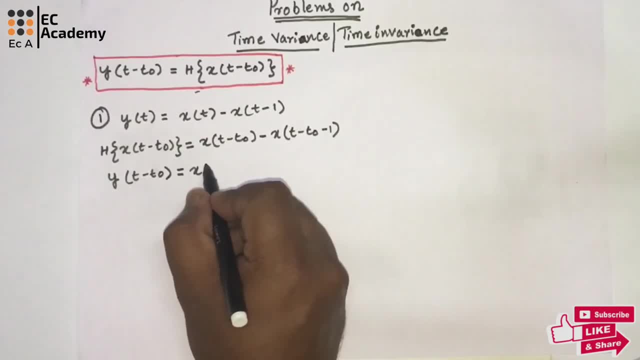 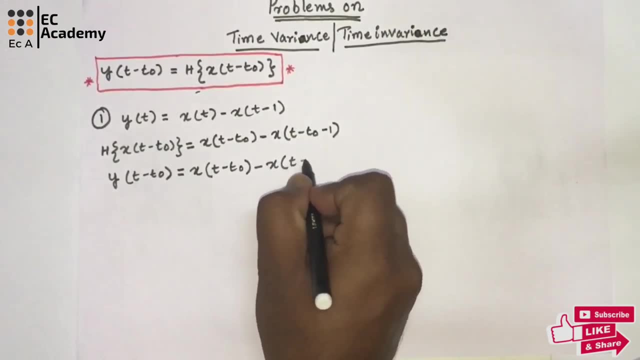 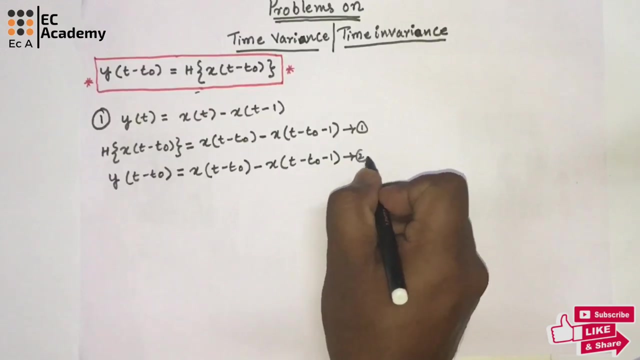 x of. so if we replace t by t0, so it will be t minus t0 minus x of t minus t0 minus 1.. So if we take this as equation 1 and if we take this as equation 2, if we compare 1 and 2, 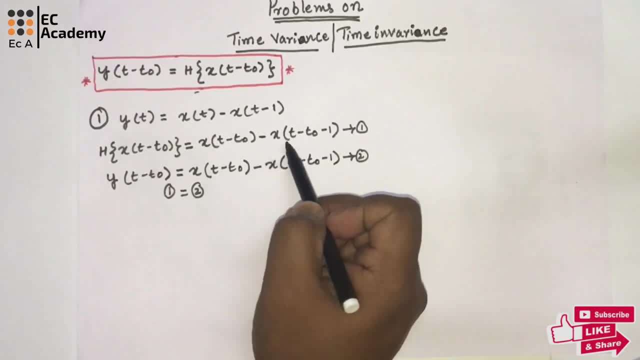 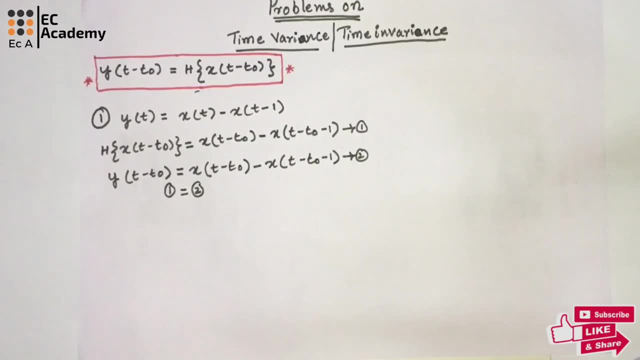 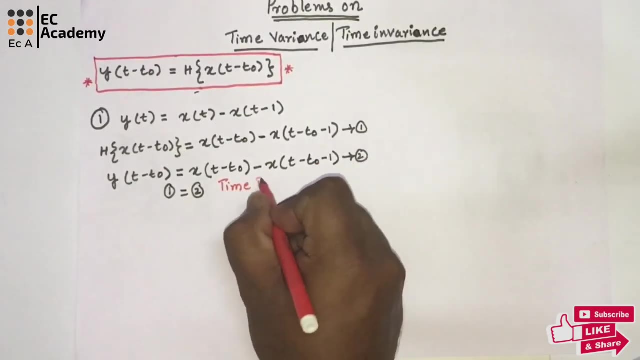 both are same, So time shift at the input is reflected at the time shift at the output. Hence we can say: the given system is time invariant system, The system is time invariant system. Let us consider the second problem, where y of n is equal to x of minus n. Now let us perform the 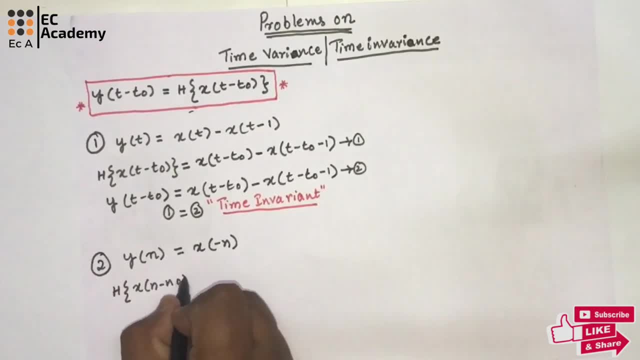 time shift at input: n minus n0.. Now to perform the time shift at the input, we need to take the equation y of n as equal to x of t minus t0 minus t0 minus. x of t0 minus t0 minus. we can write this as x of minus n minus n0.. Let us call this as equation number 1.. Now let us see. 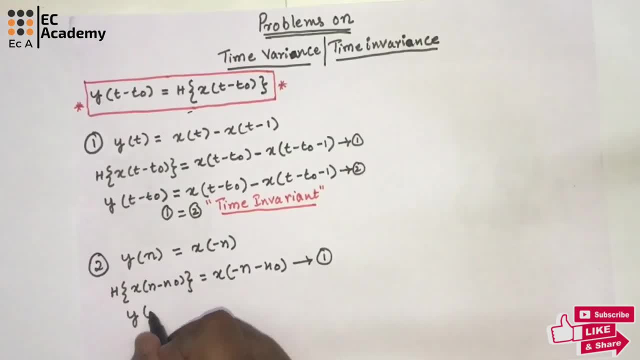 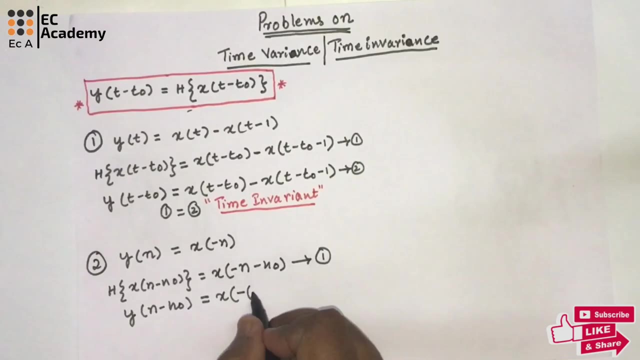 the time shift at the output y of n minus n0.. So for this, always remember, you need to replace n by n0. So if we take x of minus, we need to replace n by n0. So it will be minus of n minus n0. 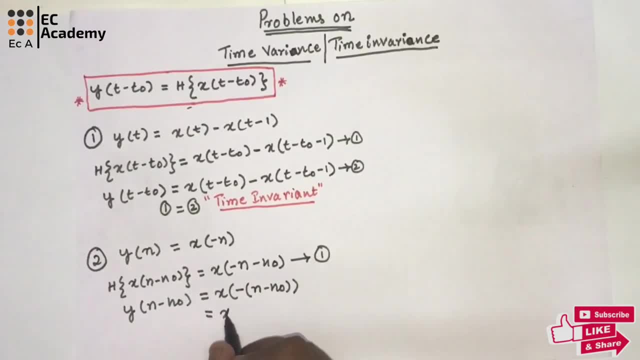 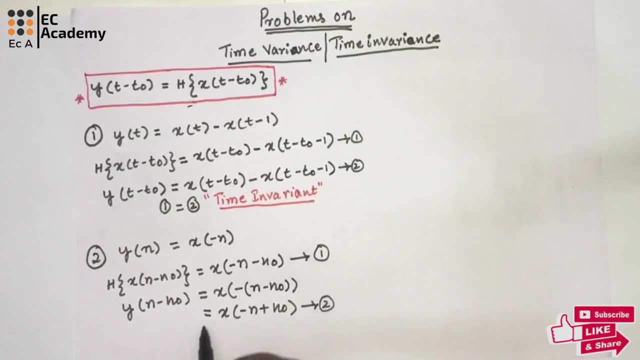 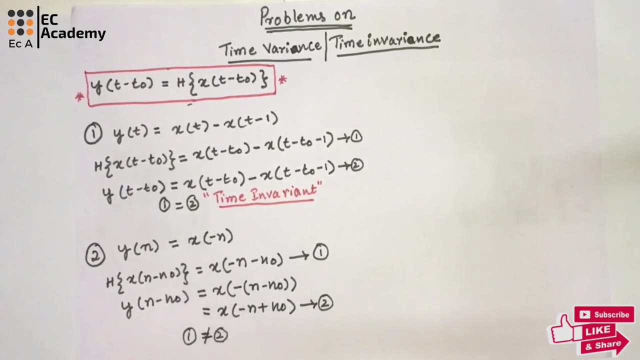 So this is equal to x of minus n plus n0.. So if we take this as equation number 2 and if we compare equation 1 with 2, both the equations are not same. That is why we can say: this system is time variant system. It is time variant system. 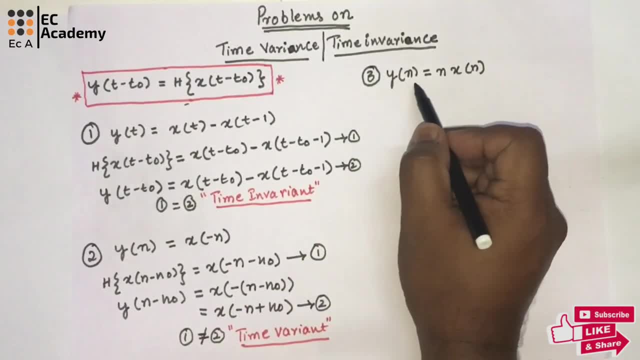 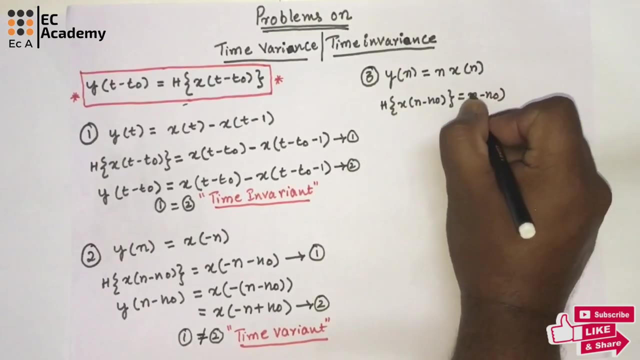 So let us consider the third problem. Here we are taking: y of n is equal to n, x of n. So now let us perform the time shift at the input, So it will be n minus n0 into x of n minus n0.. Let us take: 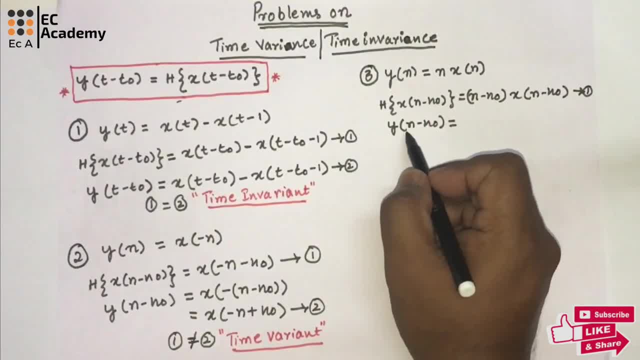 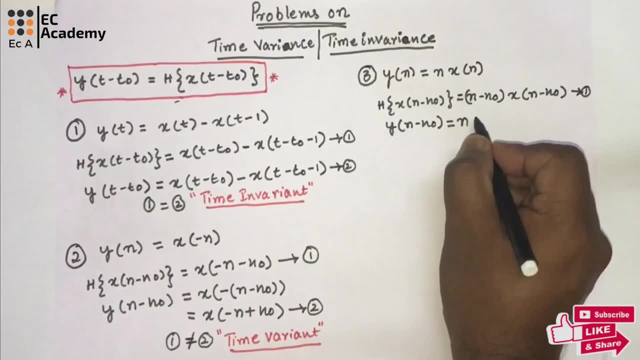 this as equation number 1.. Now let us perform the operation y of n minus n0.. So in x of n we need to replace n by n0. So it will be n of x of n minus n0.. So if we compare both the 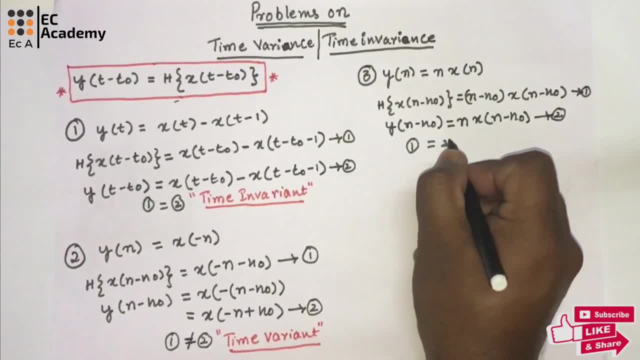 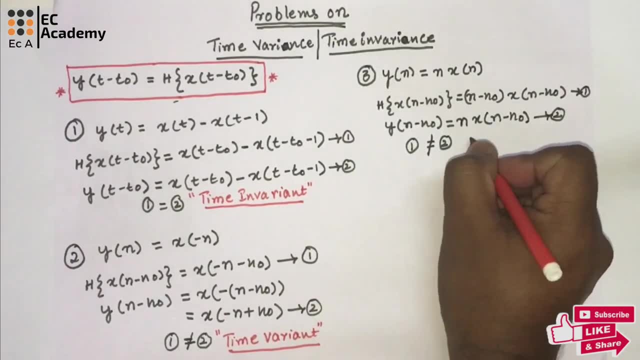 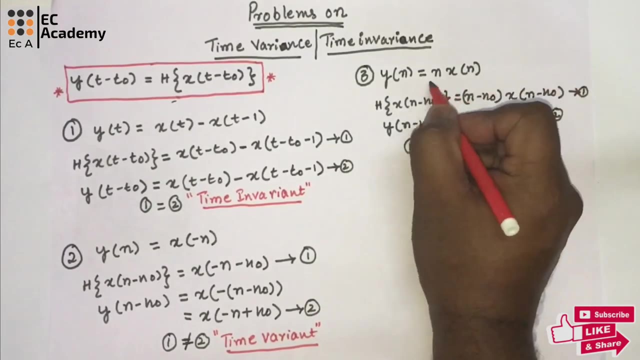 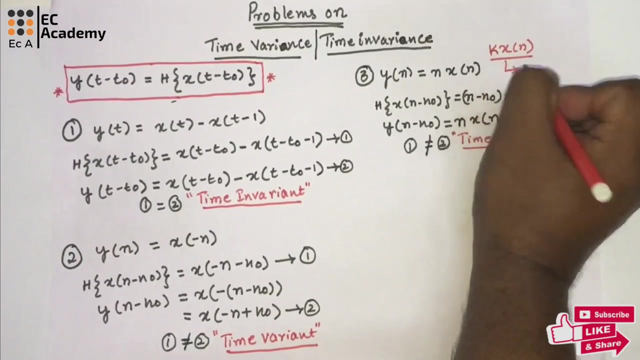 equations: equation 1 and equation 2.. So both the equations are not same. Hence we can say this system is time variant system. Similarly, instead of n, if they give any constant, let us say n. So for this the system will be time invariant. So you can solve this problem and check In place. 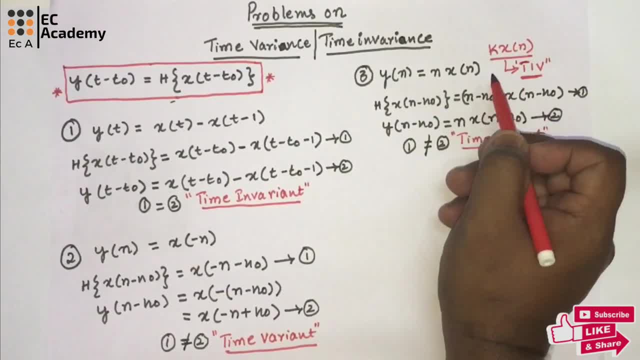 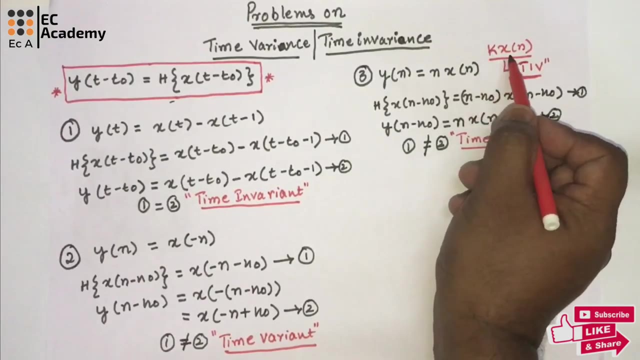 of n. if they give any constant k, let us say So, at that case this system will be time invariant system. So, since they have given n here, So the system will be time variant system. It is changing. So if you take any constant here, So we are not making any changes to this constant, We are just 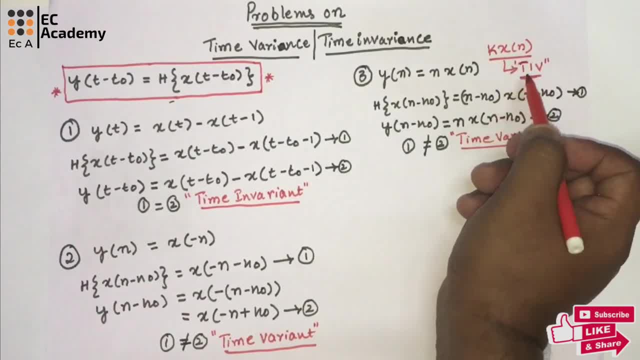 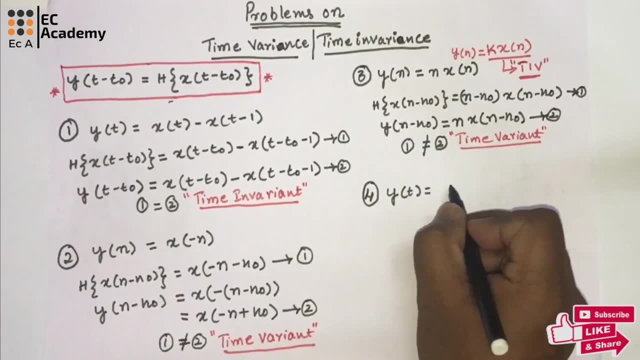 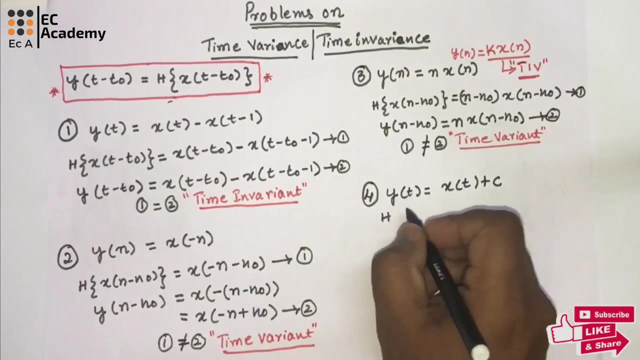 making the changes to the n which is available In x of n. That's why the system will be time invariant. Let us take y of t is equal to x of t plus c. So let us perform the time shift at the input x of t minus t0.. So it will be x of t minus. 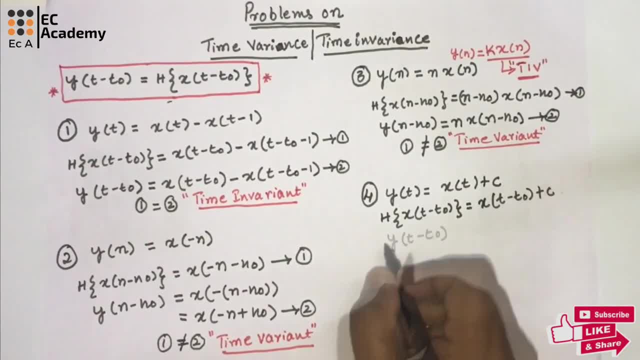 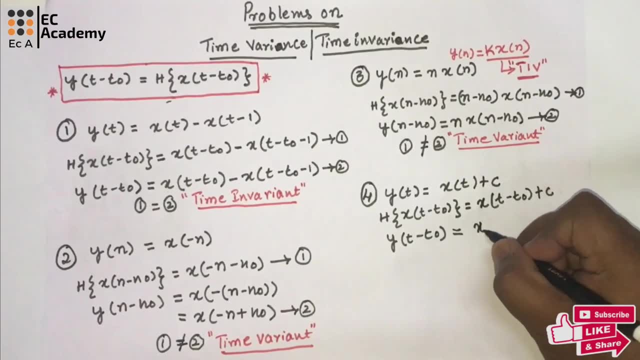 t0 plus c. Similarly, we will perform the time shift at the output y of t minus t0.. So it will be x of t minus t0 plus c. So let us consider this as equation 1 and this as equation 2.. If we compare 1 with 2, you can see. 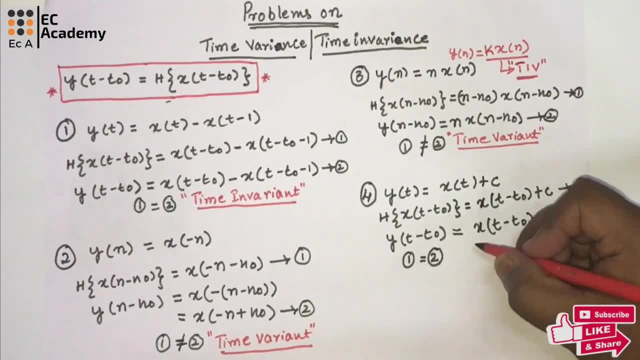 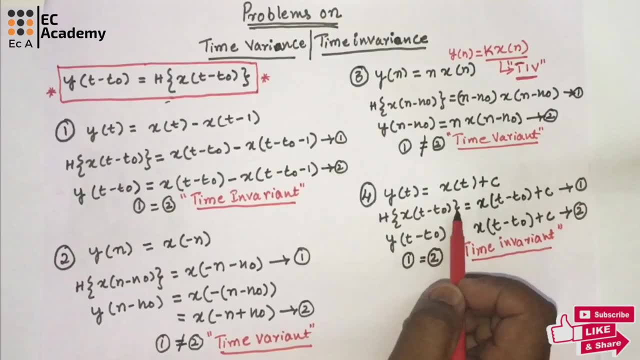 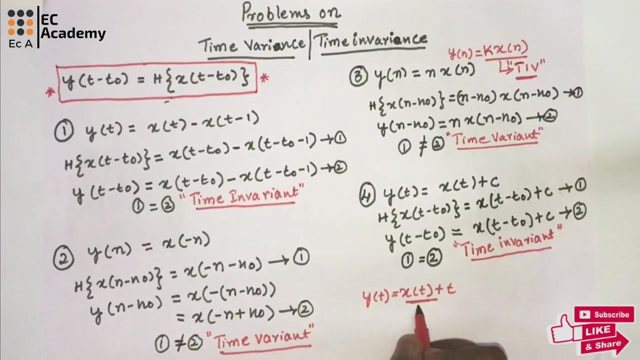 both the equations are same. That's why we can say: the given system is time invariant system. So in the same problem, if we take instead of c, if we take t, x of t plus t, So if we take y of t is equal to x of t plus t. For this the system will be time invariant system. So you can solve this. 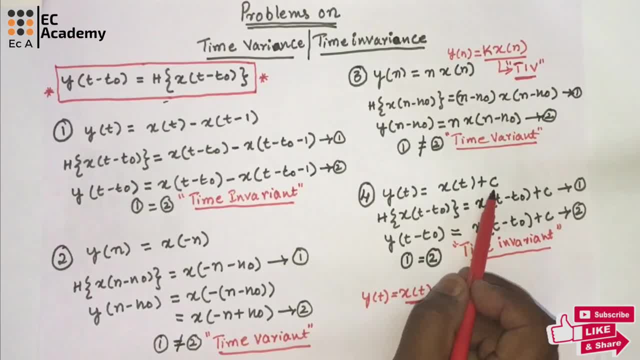 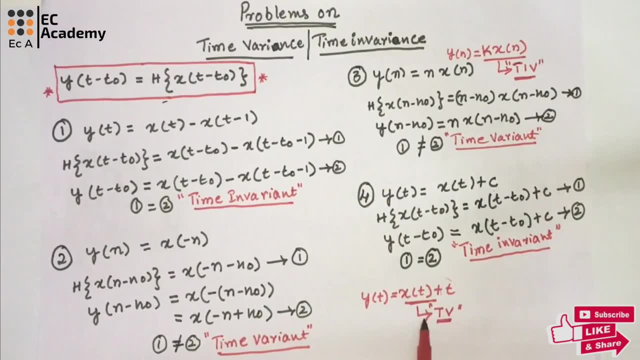 problem and check. So in this problem we are having some constant c, So that's why it is time invariant system. We are not making any changes to this. So in this problem we are having x of t plus t, So we will get time variant system. So this is about.